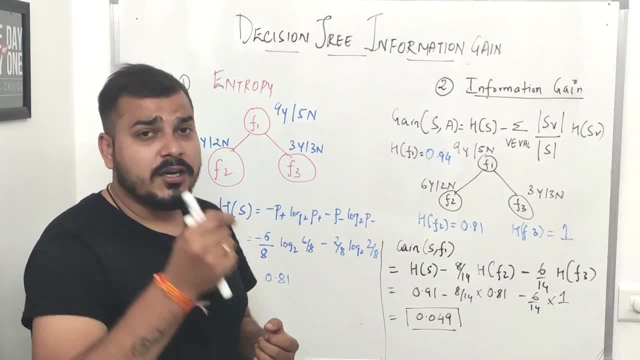 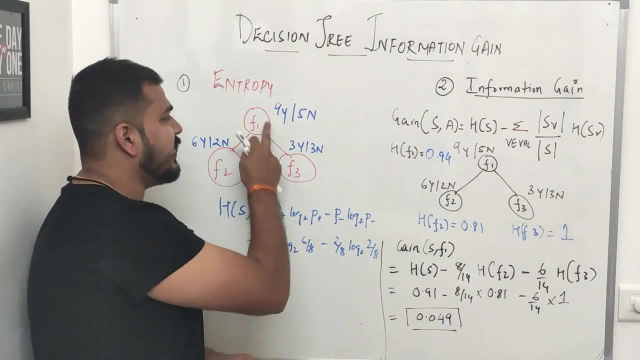 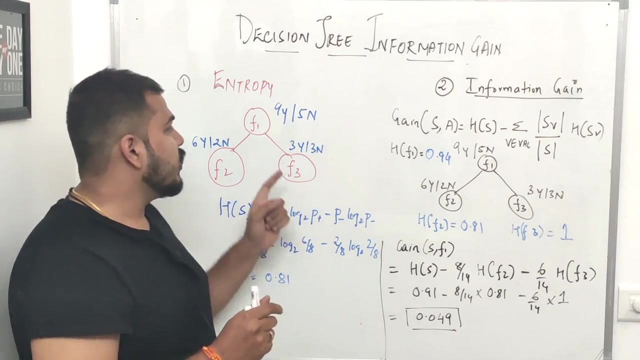 going to revise a quick revision about entropy itself. so entropy actually helps you to calculate the purity of a subset. now what does this purity actually mean? understand, guys, in decision tree we consider features and then we divide those features. you know, divide those features based on the output. now suppose i'm considering feature one. okay, suppose i have cons. i have in my machine. 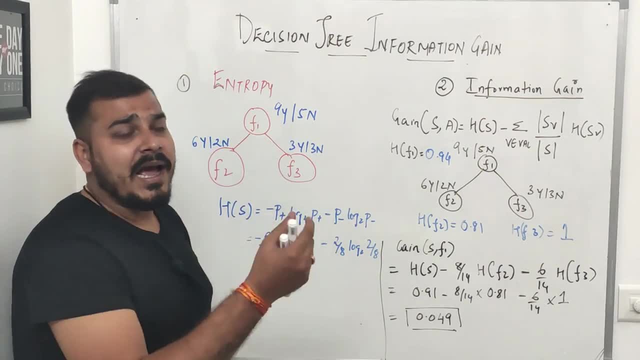 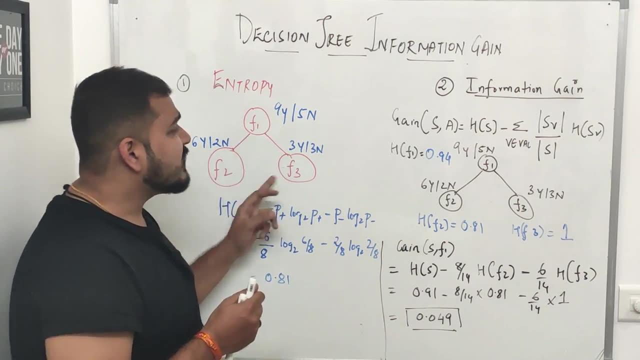 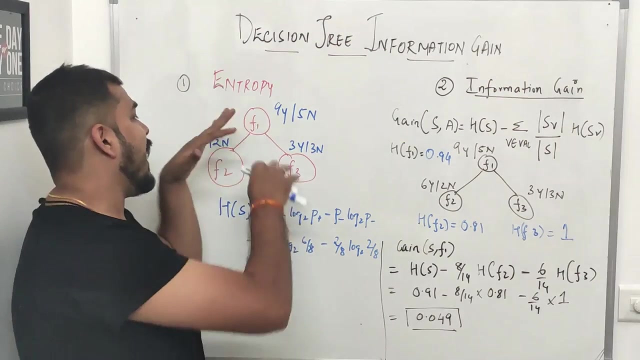 learning problem statement. i have three features- f1, f2 and f3- and i have an output variable which has, like yes or no, a simple binary classification. okay. now, when i'm considering this specific example, suppose for the feature one, i have total number of nine yes and five no's. okay. and when i split it, 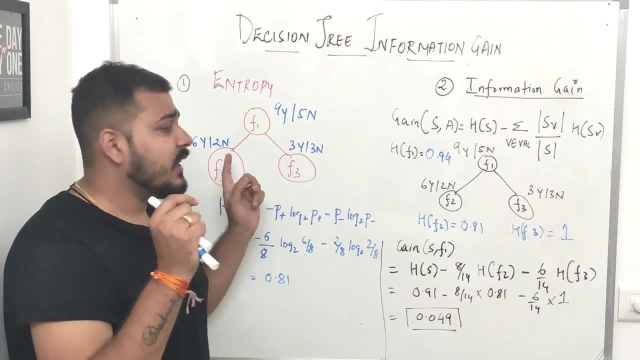 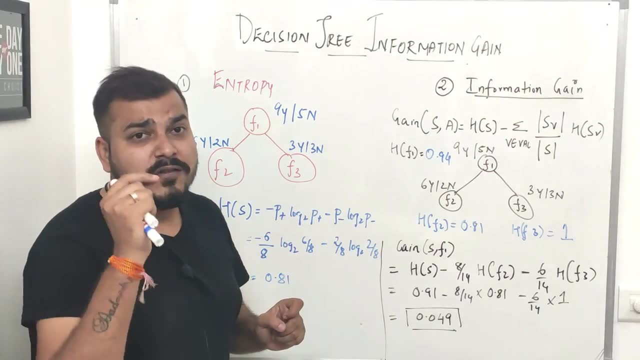 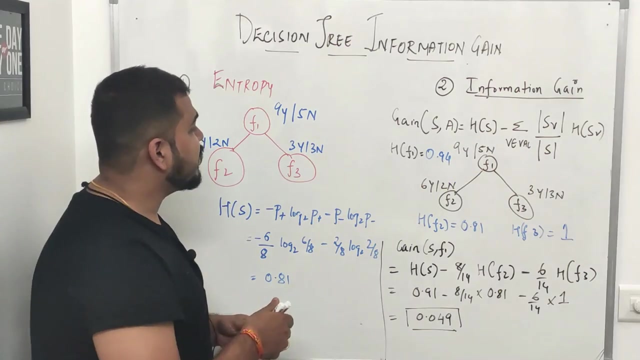 okay, suppose i'm splitting based on f2 feature and here i'm getting six yes and two no's output, and over here i have f3, which is 3s and 3 no's. now one of the thing is that this splitting will be going on unless and until we get a pure subset. now what is exactly pure subset? pure subset is: 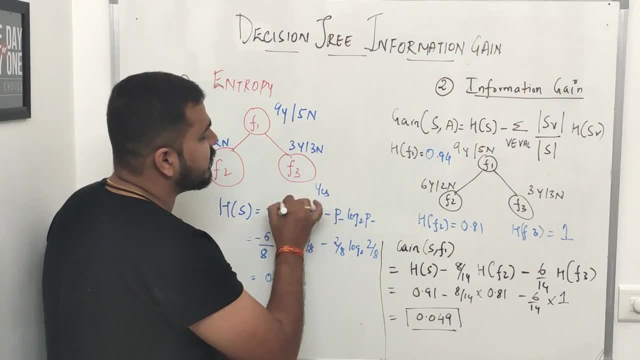 a situation where i get either completely yes or i get completely no. okay, so that basically means i should either get, uh, all the yes, suppose, over here in this particular scenario i have three. In this particular scenario I have like two nodes, only that Specific number, and this is basically called the leaf node. Okay, so in that specific way, 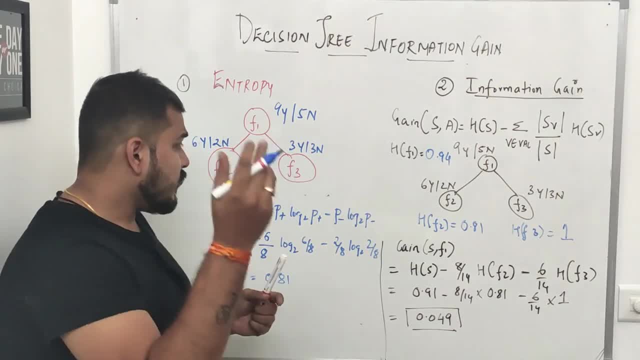 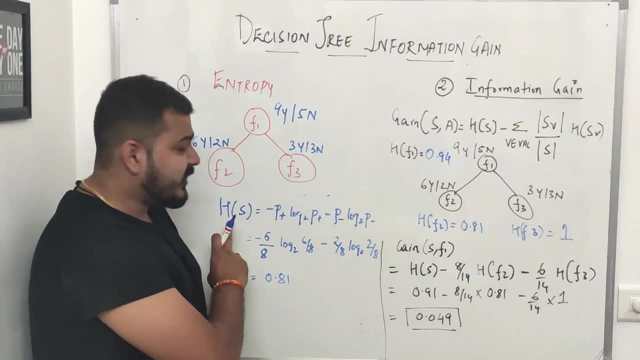 I am actually calculating the purity of the sub split. Now, if the split, if the feature based on this. now suppose, if I take an example, The entropy formula is given as H of s Minus, P of plus. I'll explain you about this particular variable. I have also explained in my previous variable. 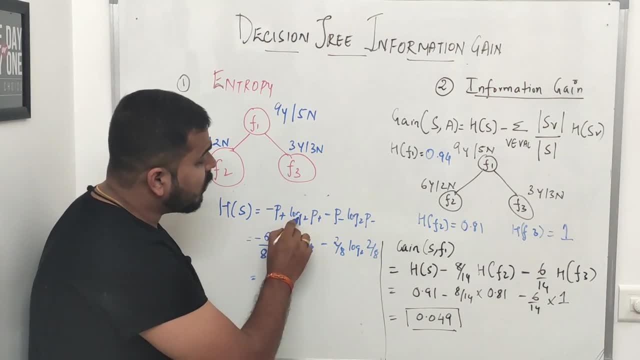 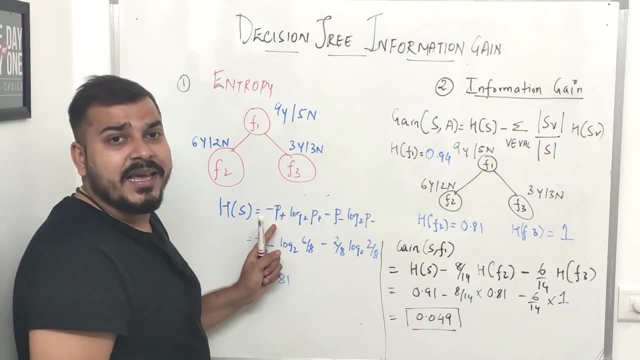 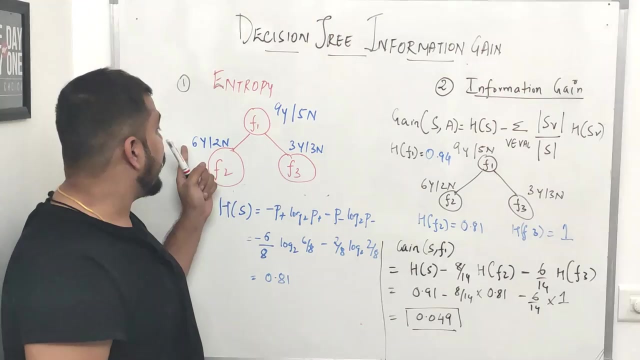 Previous video. sorry, so minus P of plus: log to the base 2 P of plus. minus P minus: Log to the base 2 P minus. now What does this particular formula say? P of plus is basically when I am doing the split, suppose I do the split on, based on f2.. Okay, how many total number of yes I have got okay. 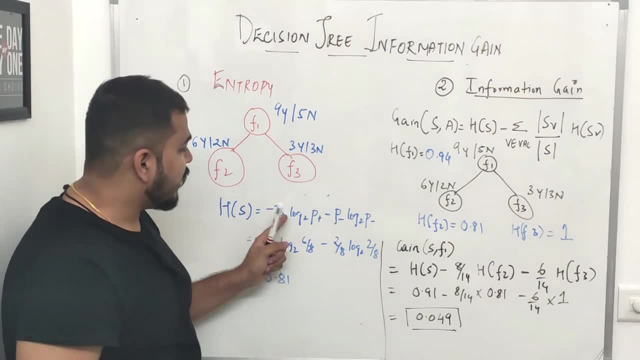 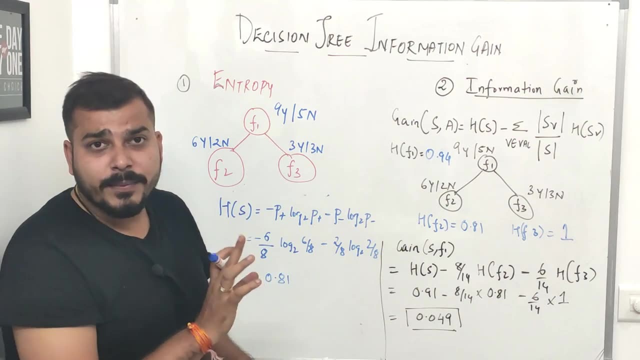 How? what is the percentage of total Yes that I have got now in this particular scenario, if I want to find out on f2, if I am calculating the purity split of The f2, which is actually determined by entropy In this particular scenario I have sixth s and to know now if I want to calculate P plus. 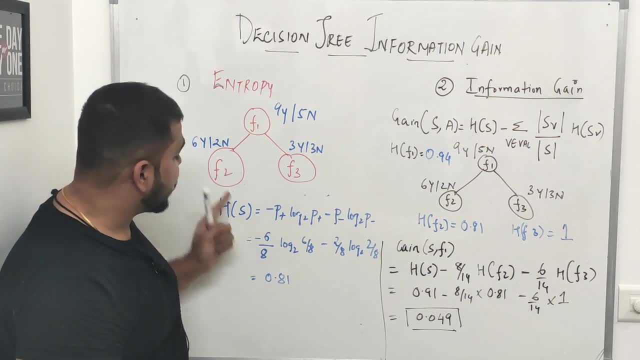 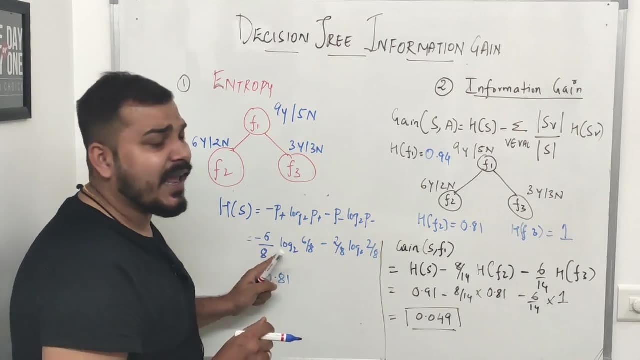 That is the percentage of positive values. So I am going to take 6 divided by 8. Okay, 6 divided by 8?? Why 6, 6, 6, total number of yes. then I'm dividing it by it because I told people asses. 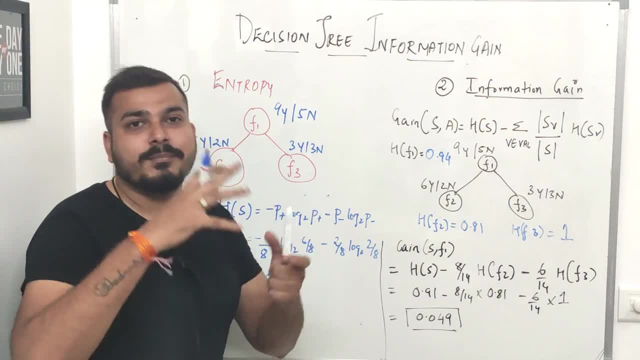 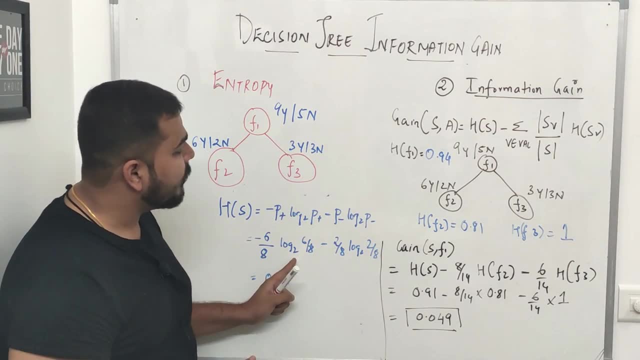 percentage of positive values. When I want to calculate the percentage of positive value I also have to take the total number of knows also write together. So here I am writing at 6 by 8. log to the base, to again: P of plus is there. I'm going to take it to the right Dan PDF right now if I don't have enough line range right, so here. 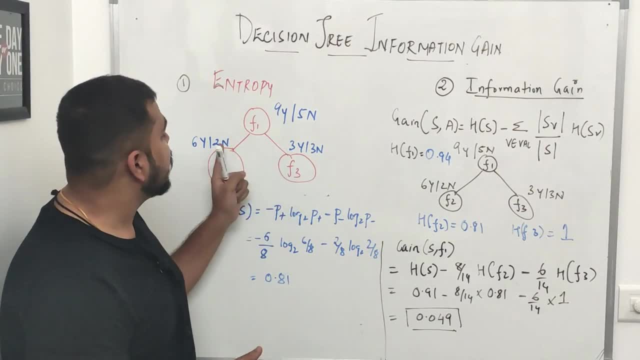 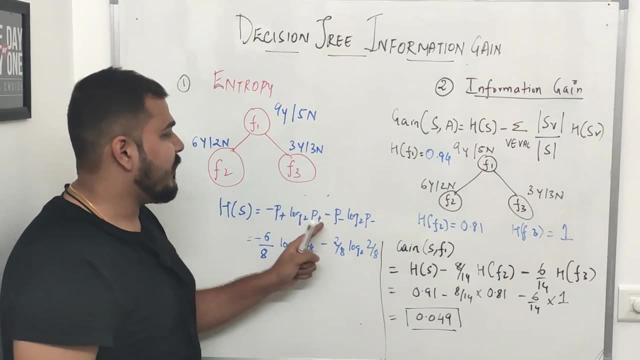 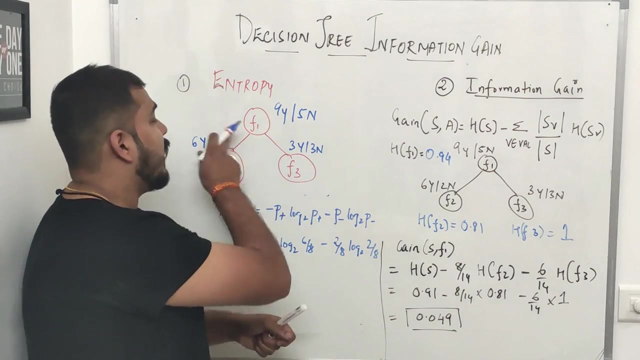 6 by 8 minus. what is p minus? now p minus in this particular scenario, right is 2, right 2? no's are there. so i'm going to calculate the percentage of negative values. now p minus. okay, so 2 divided by 8, log base 2. 2 divided by 8, again 8 will be same, because that is the total values. total dependent. 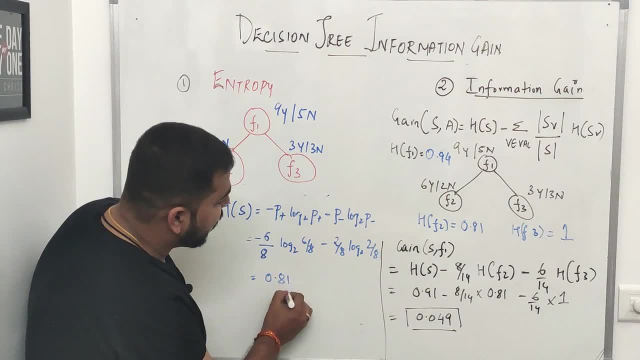 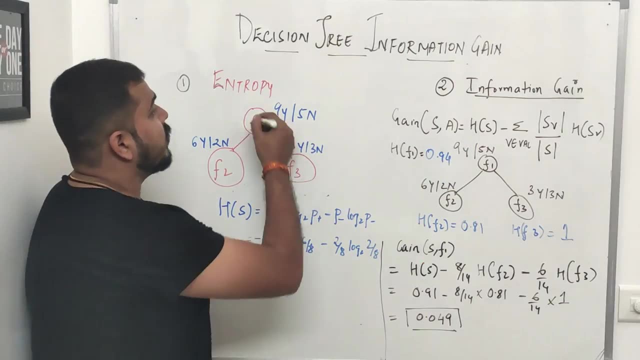 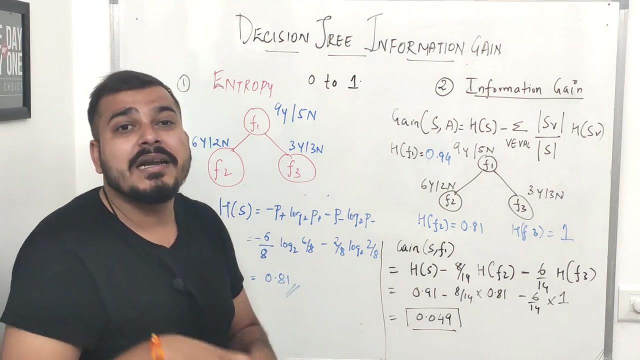 variables that i've actually and when i actually compute it, i'm actually getting 0.81. okay, 0.81. now also, remember, guys, which i have also mentioned in my previous video: the entropy value, the purity value, ranges between 0 to 1. 1 basically says that it is a completely impure subset. now, impure subset. 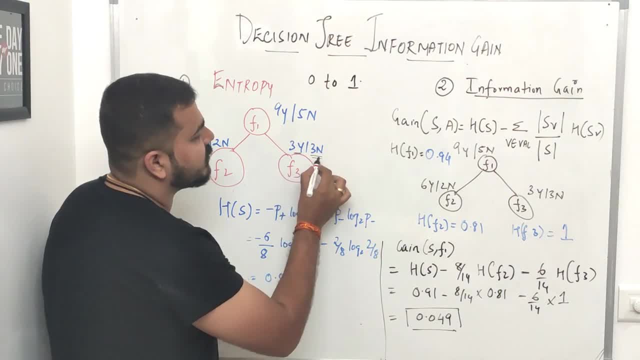 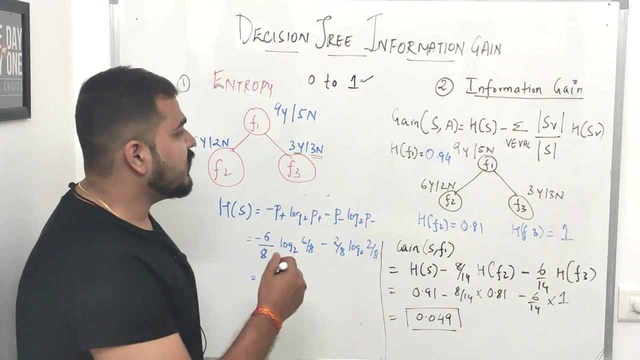 basically means that suppose i have 50 percentage of yes and 50 percentage of no. in this scenario, if i apply this particular formula right, i will be getting the entropy value as 1. now suppose if i have a leaf node where i have like 5 yes and 0 no's, this is a leaf node. 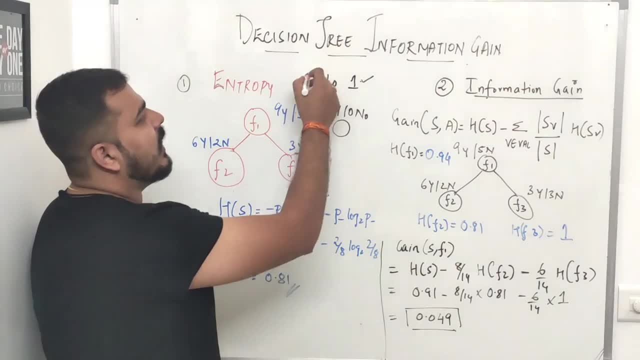 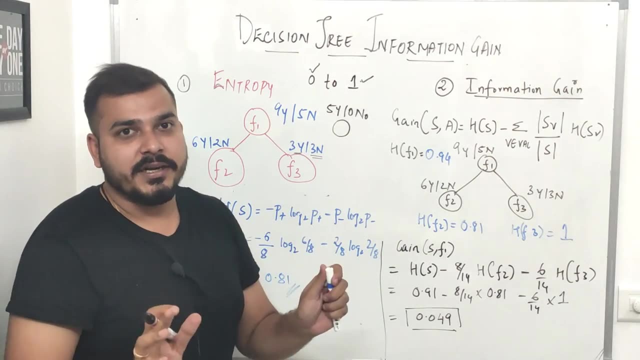 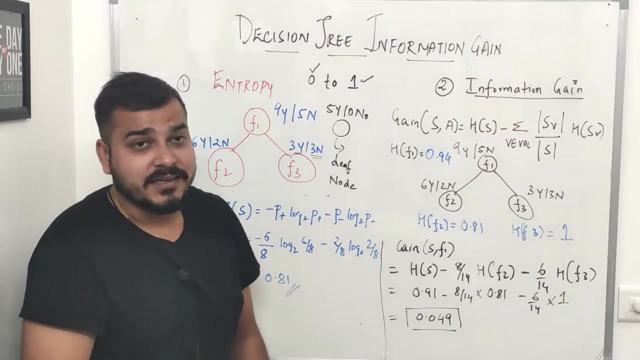 right in this scenario. if i try to apply this particular formula, i'll be getting the value as 0. and now, when i get the value as 0, at that time i have to stop splitting in decision tree, because this is actually my leaf node. this is my leaf node, okay. so i hope you are understanding this. 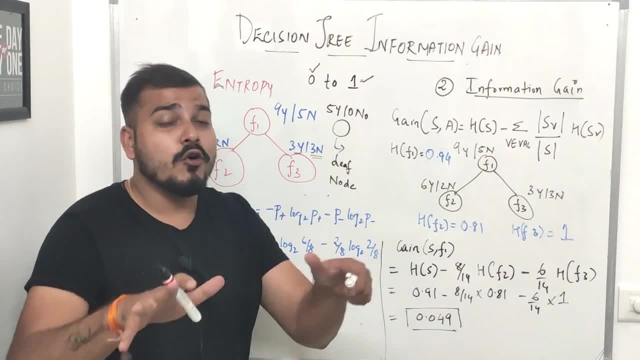 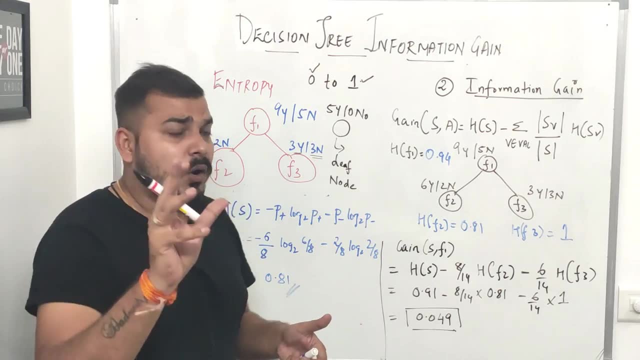 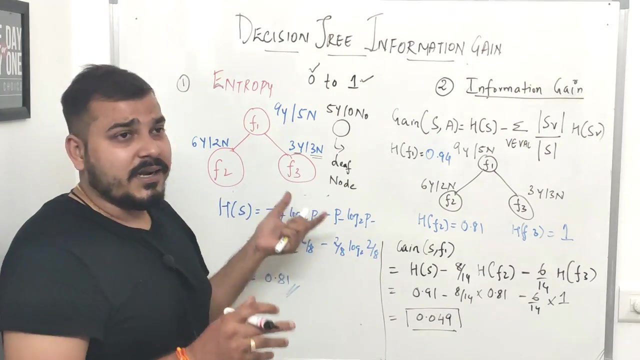 and we have to stop. usually decision trees, all the splitting happens for overfitting condition. we actually get a pure subsplit at the end. okay, this is basically my leaf node. now, understand one thing: in entropy we are just getting whether the split is pure or not. but understand guys, in a decision tree we 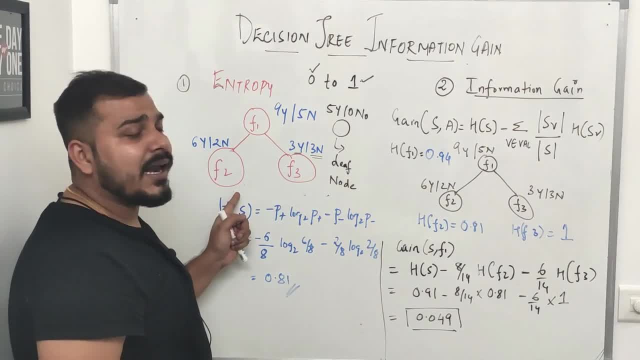 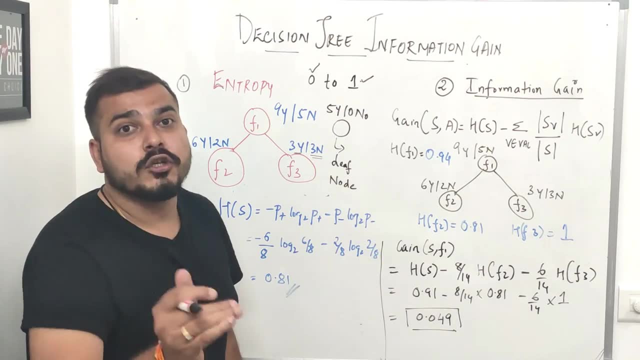 have to take many number of features like this. suppose i am splitting over here as f2, here as f3. i need to again split with some other features continuously till i get the decision tree. so which pattern should i select? should i go with first f1, f2, f3, or i can also go with f1, f3, f2 right in? 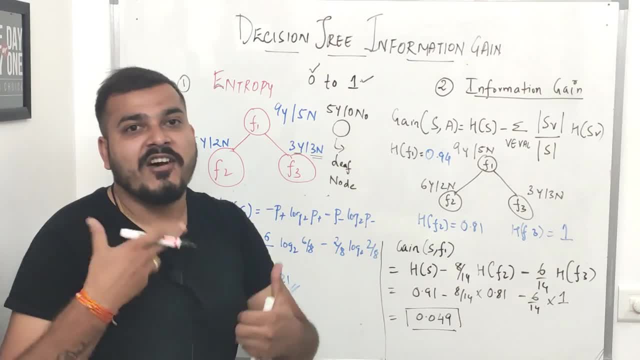 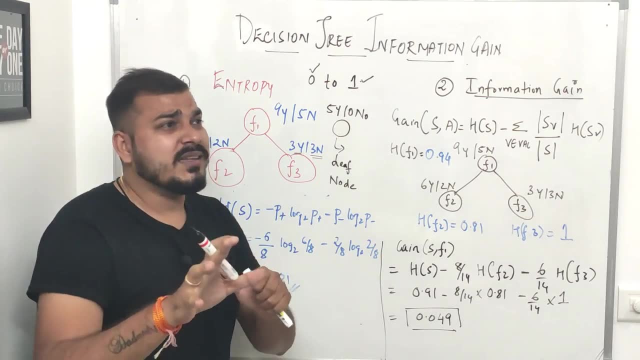 that particular way. also, i can go, but how do we compute that? how do we find out? so, for that specific split, we use something called as information gain. now, what is information gain is that? in short, you can say that i am going to compute the average of all the entropy. okay, i am going to compute the 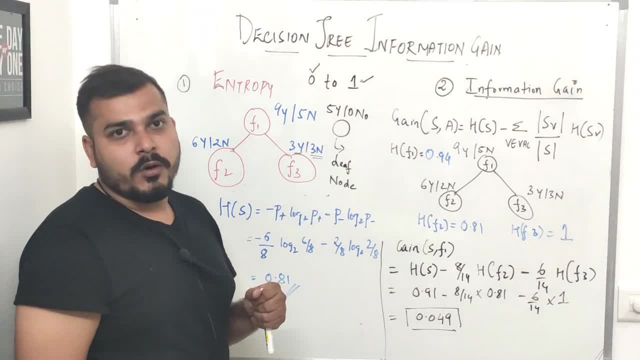 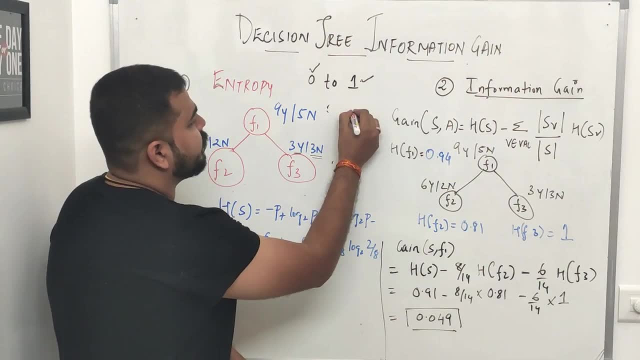 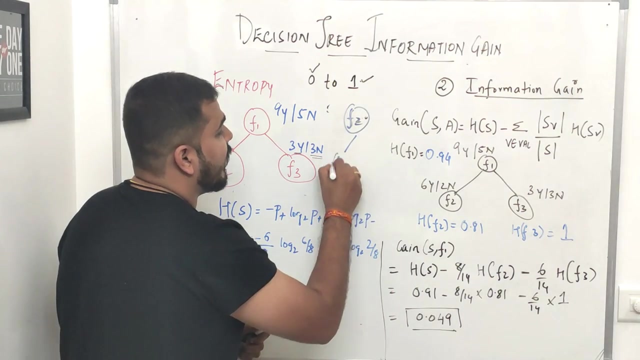 average of all the entropy based on this specific split. okay, suppose i have one more scenario where i am actually, instead of this, what i am doing is that i will just use another split, suppose i am going to just use. okay, so here is my f2 now, based on f2, i want to make a split of f1 and 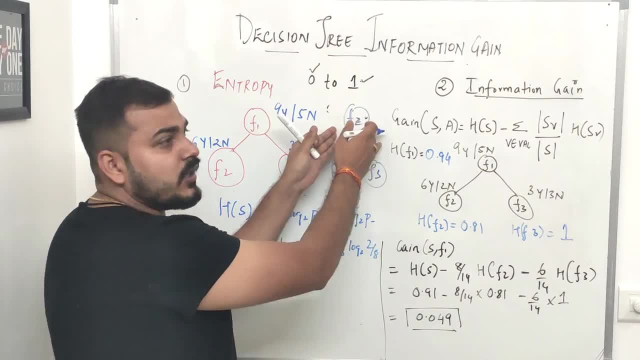 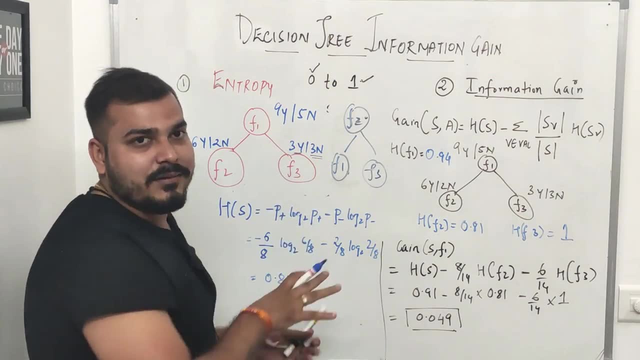 f3. now i need to understand whether this split is better or this split is better, and for this i have to combine the entropy of all the values right. i cannot just depend on just one one split itself. so for that we actually compute the information gain. now, information gain: what does? 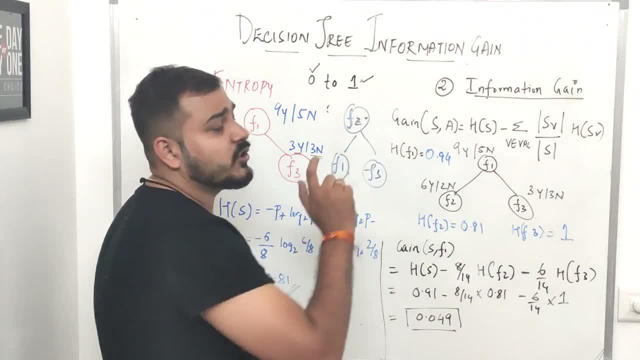 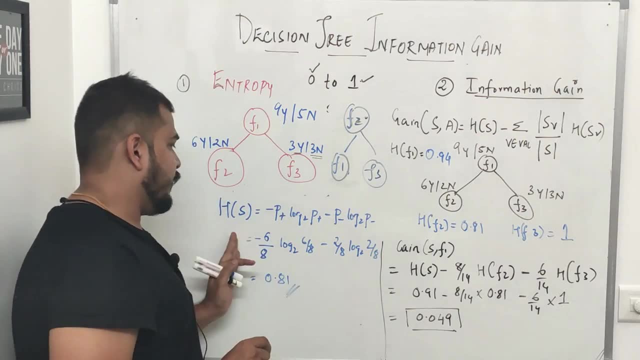 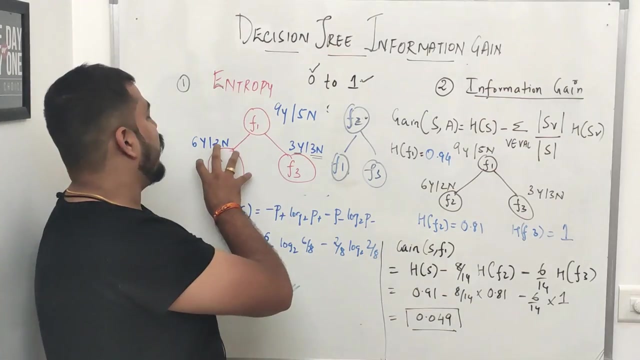 it, do the formula. please note down this particular formula. it is pretty much important. and the gain of s, comma a is equal to h of s. h of s is basically the entropy. okay, this entropy, uh, for this specific split. okay, suppose i want to calculate the entropy of this. i want to calculate the entropy of this. 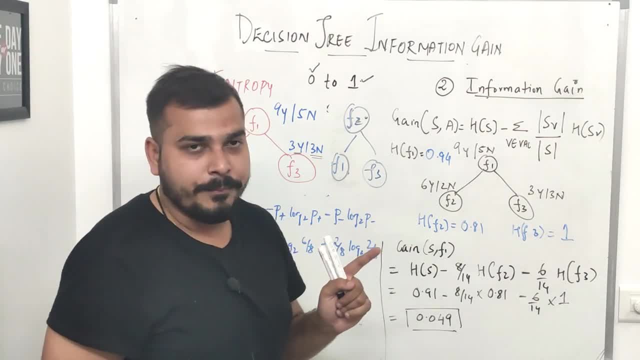 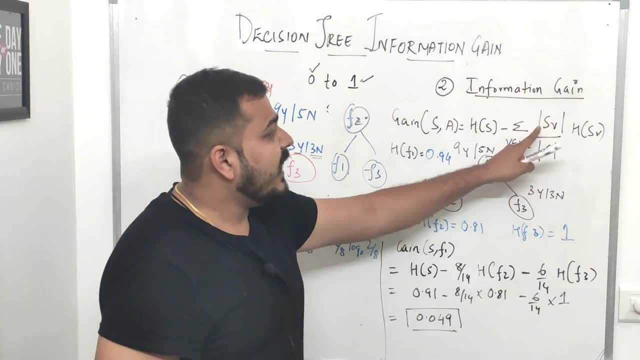 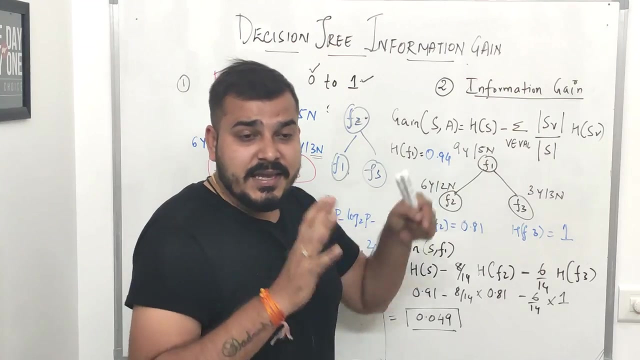 i want to calculate the entropy of this. that is what h of s actually mean. then, minus summation of v, two values. i'll just explain you what is this values? then this is s of v. and remember guys, s is basically the subset. okay, s is basically the subset. s of v is actually the subset after. 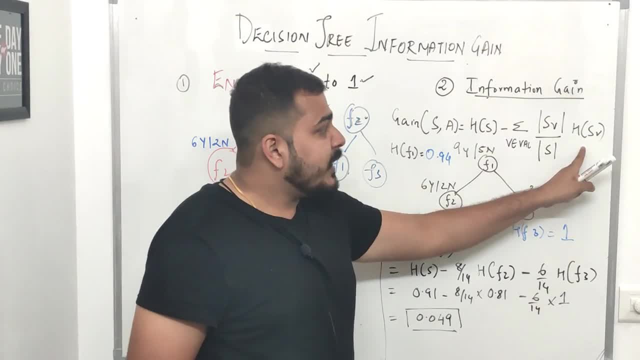 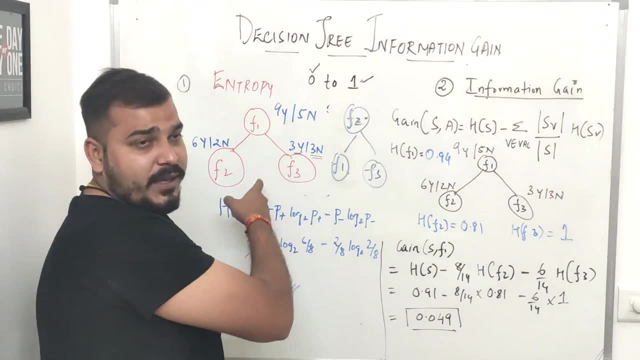 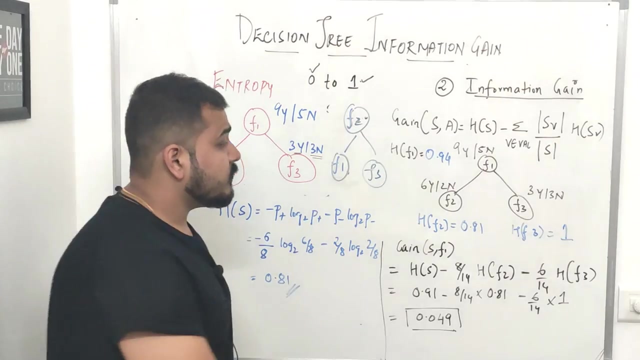 splitting. okay, and this is total subset multiplied by h of sv. h of sv basically means, after the splitting, i want to calculate the subset entropy. so that is what this h of s? v actually means and you'll understand this. this formula looks a little bit complicated, but when i'm computing it, you'll understand it pretty much easily. okay, let us go ahead and try. 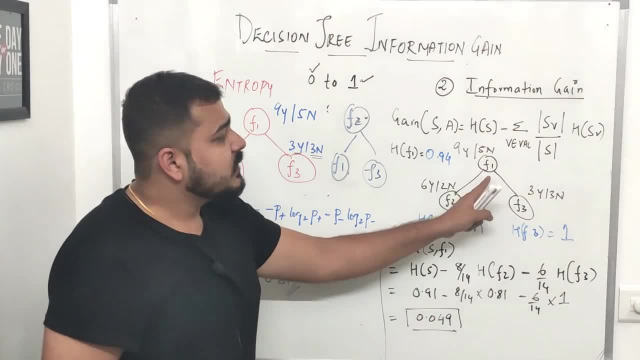 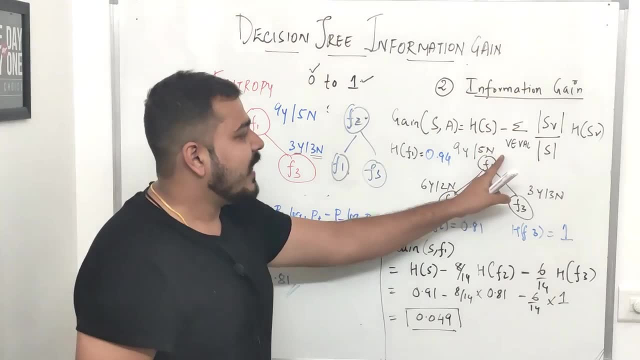 to understand. now suppose i have a split over here. this is f1. i'm splitting it based on f2 and f3 and same problem statement i've taken here. initially i had 9y 5, nos 6s, 2, nos 3y 3, nos. 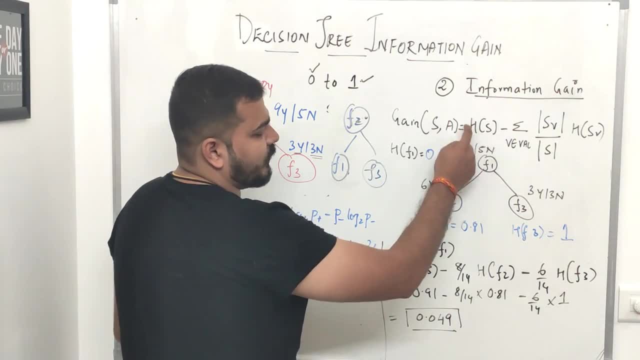 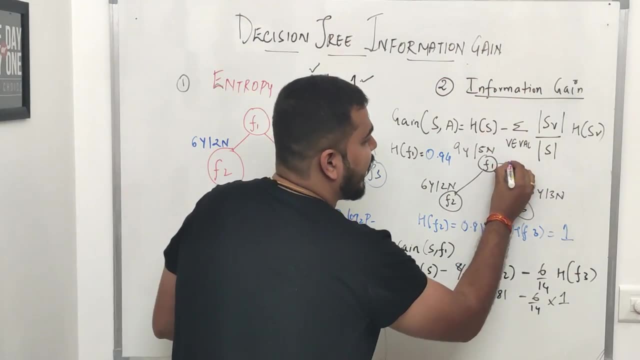 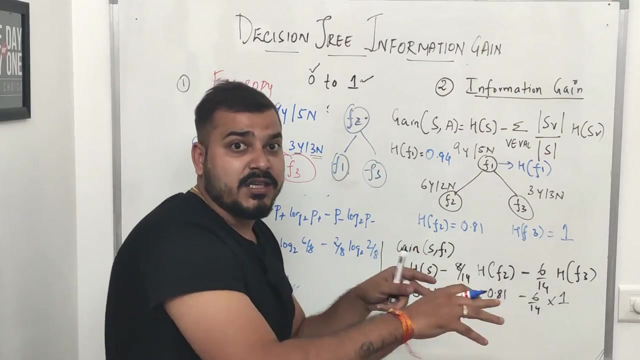 now the first step in this: i have to compute h of s. okay, i have to actually compute h of s. h of s is basically for this subset. specifically, i'm going to take h of f1. is my h of s? okay, because, understand, this is this: h of sv is after the split. after the split, what is the entropy? h of s is for. 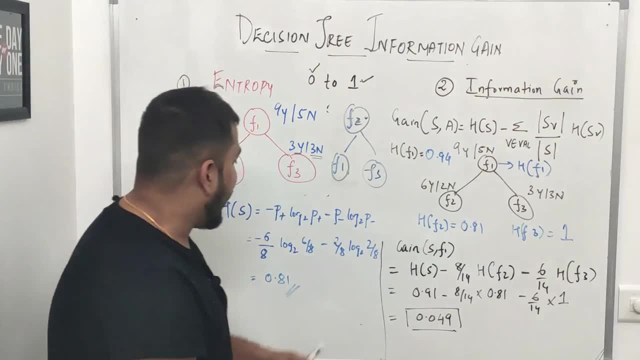 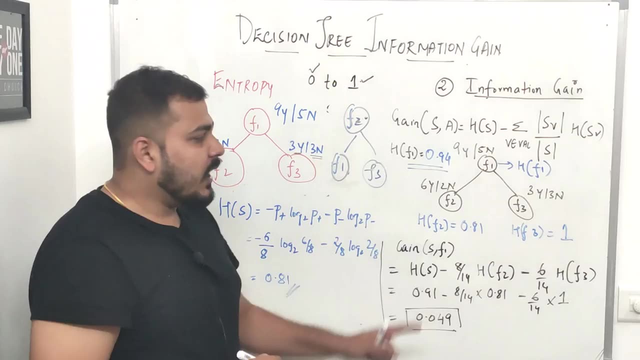 the root node. okay, so i, if i compute h of f1, i'm just going to apply this same formula and for that you just do the computation. i've already done it. i'm getting. the value is 0.9. now for this h of f2, if i'm doing the computation, my entropy is coming as 0.81. again the same. 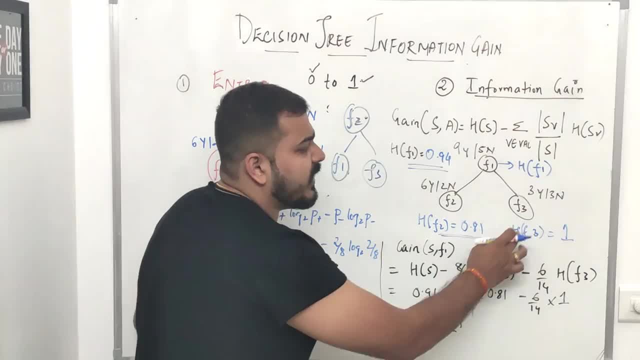 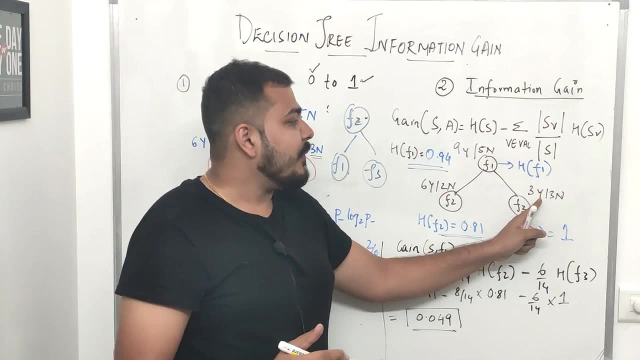 formula: nothing, no change in that. okay then, f of 3, h of f3. when i'm finding out, my entropy is coming as 1. why 1? because this is a pure impure split. right, because i'm getting 50 percent of yes and 50 percent of no, and i told you the value ranges between 0 to 1 if it is completely impure. 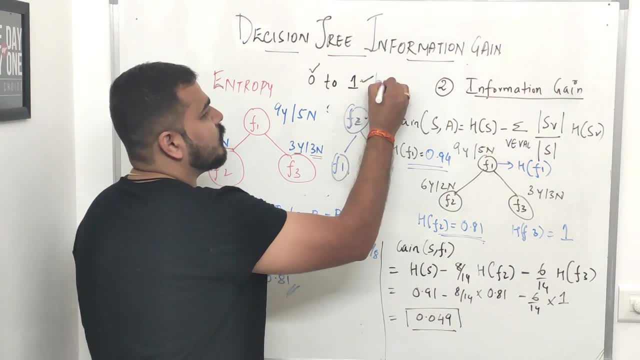 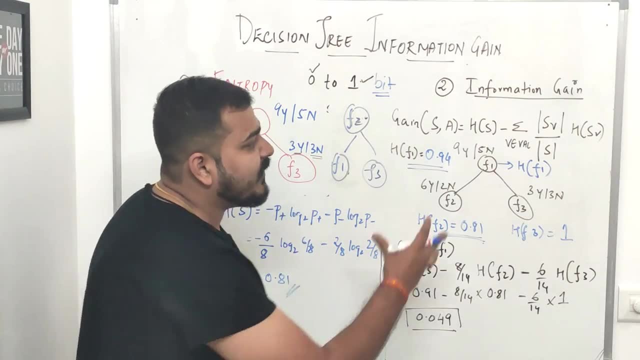 i'm going to get as one value one bit. we'll basically say this as bit: okay, if it is a pure split, it is a pure split. okay, if it is a pure split, it is a pure split. okay, if it is a pure split, is going to get it as the value is going to come as 0 bit. okay, now i have calculated this. h of f. 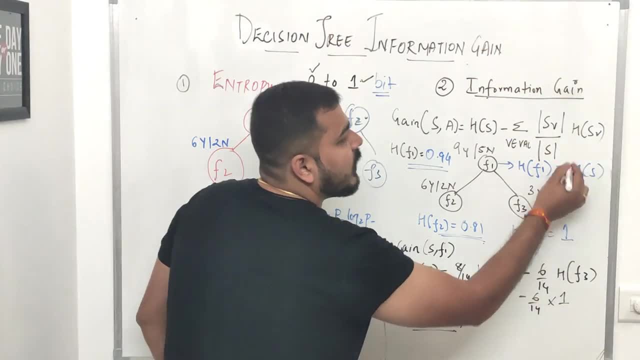 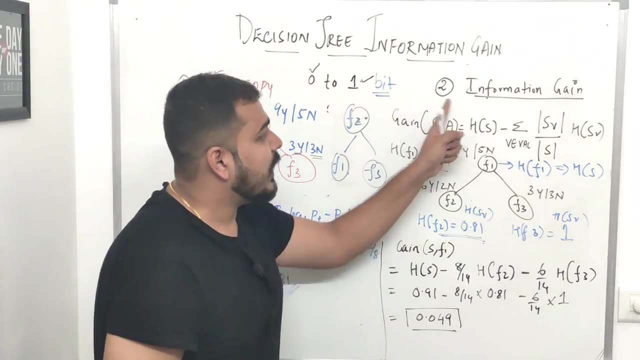 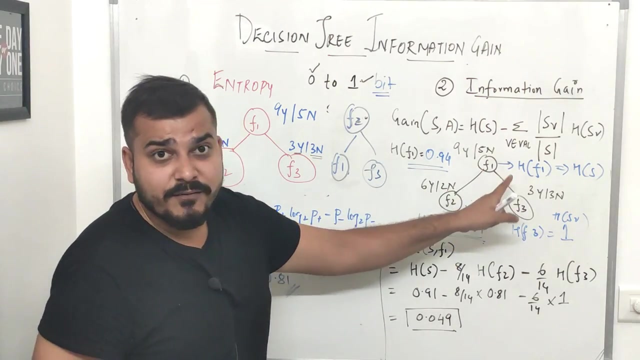 this is basically just like my h of h of s. this h of sv is this one. okay, and this is also my h of sv. now see, focus on this- how i'm going to replace in this particular formula: okay, now, gain of s comma f1. okay, because i'm computing from the root node f1. so first is my h of s minus. understand this. 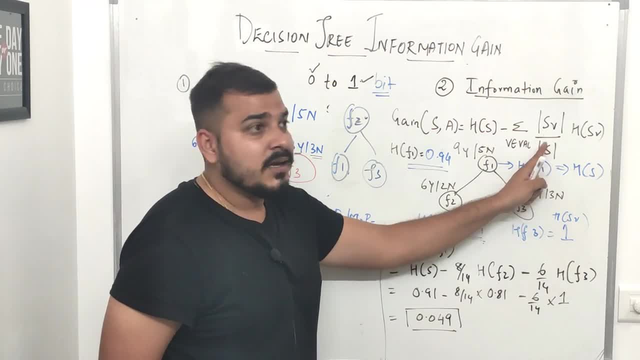 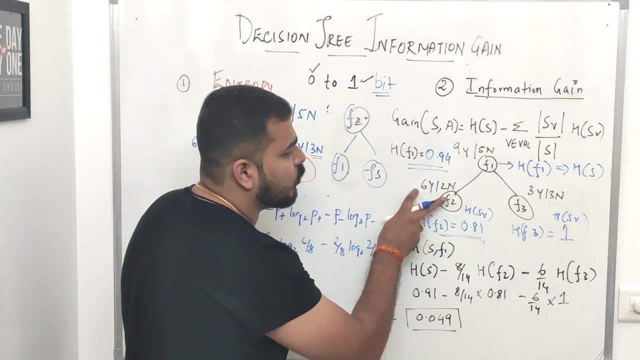 s of v divided by s. this is my total sample. this is my sample after the split. okay, now, after the split of f1 in my f2, understand what is the total number of values that i'm getting: 8, 6 plus 2, 8. so i'm going to say 8. 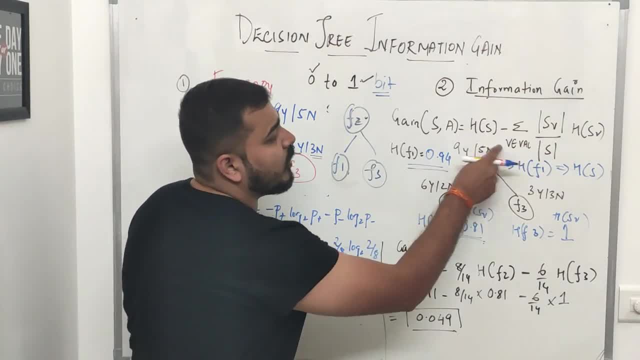 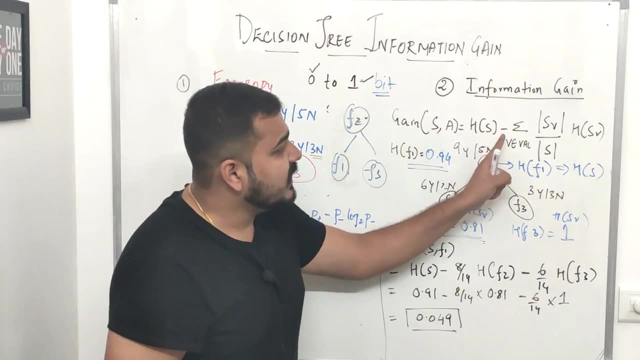 which is my s of v, divided by 14, the total number of subset. okay, so 8 by 14. h of f2: h of f2 is basically my entropy of f2, then minus. see i'm doing summation right. so minus when i'm doing. 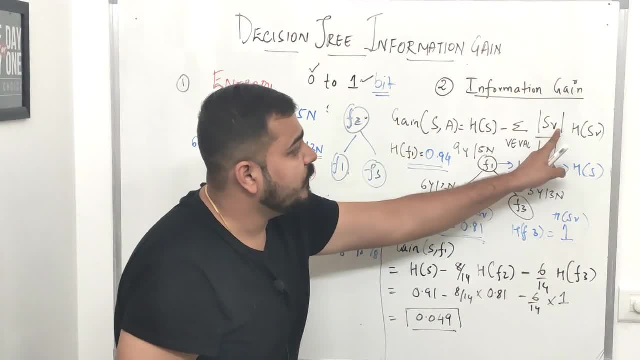 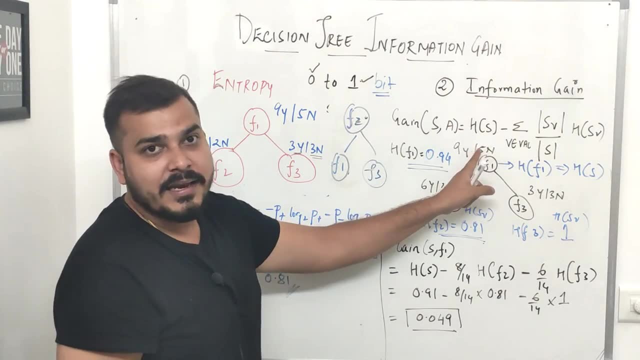 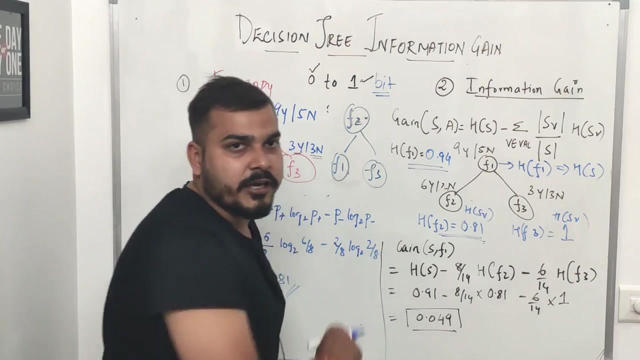 summation, this will also become minus right. and then i'm going to say: h of f2 is basically my s of v for this feature. 3 is total value 6, 6 divided by 14, why 14? my total sample is 14, 9 years and 5 no. then multiplied by h of f3, pretty much simple. okay, this is again entropy of f3. 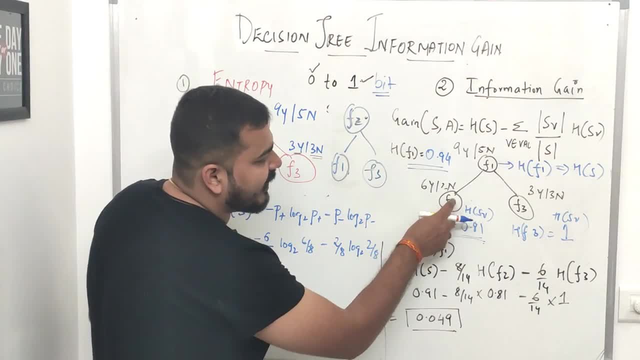 now all i have to replace is h of f2. i have computed my h of f2. this is 0.81. i'm replacing over here h of f3. i know this is the impure subset, so my value is going to be one bit. 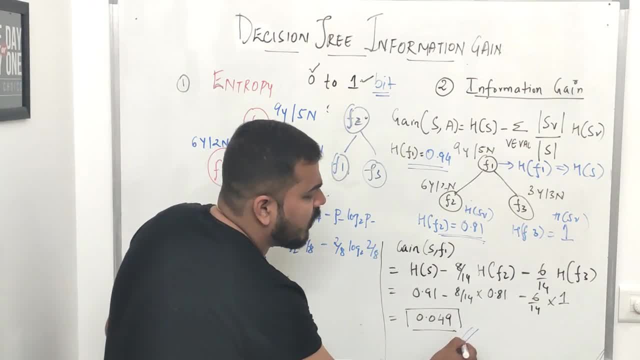 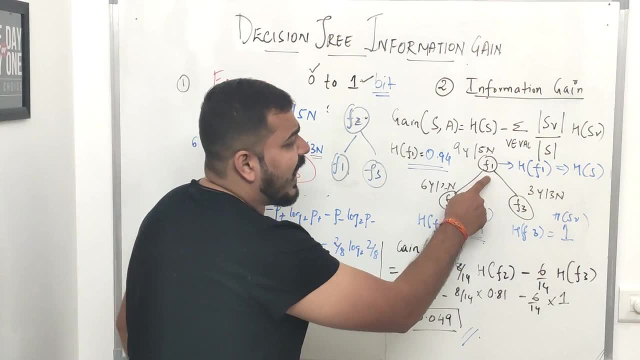 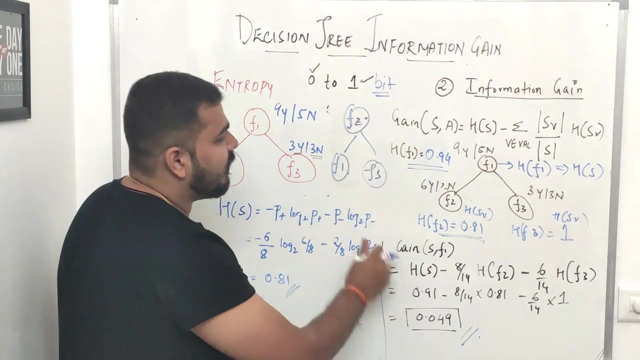 now, when i'm doing this overall computation, i'm getting it as 4- 9. now, what does this value indicate? now, here you can see that i have done f1 and i have splitted based on f2. f3 instead, i can also go with f2 and i can calculate this whole value, f1 and f3. 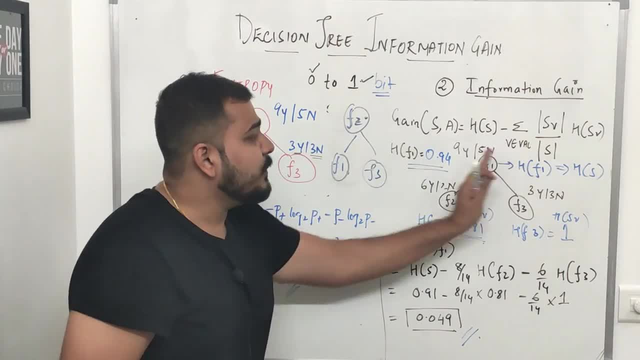 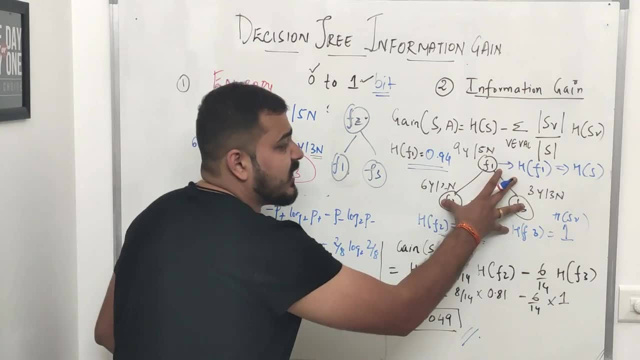 suppose, if i take these two examples and suppose which one is the perfect split that i should use in my decision tree, the machine learning algorithm will actually calculate the information gain. suppose this gives the highest information gain value, then this particular structure will actually be used in order to split the. 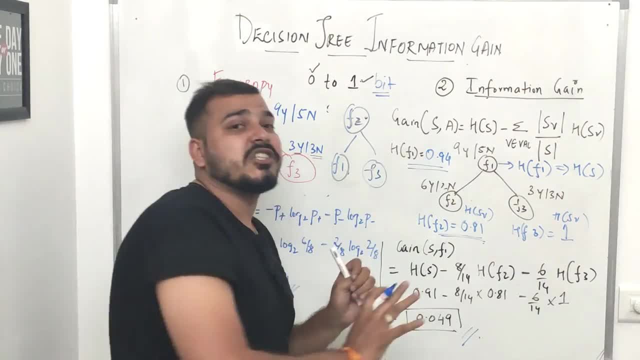 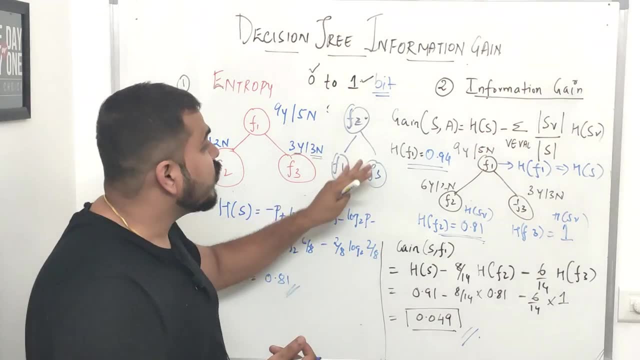 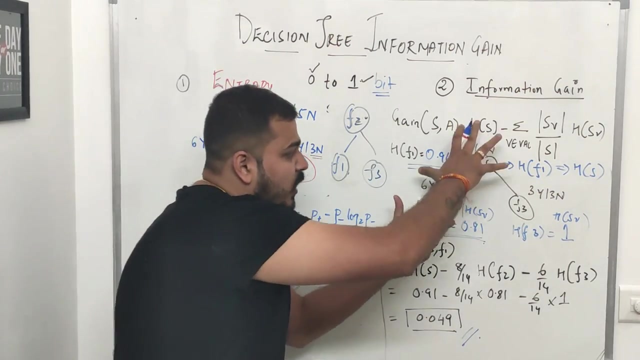 that particular data set itself in order to construct the decision tree. suppose, if this particular splitting mechanism is actually giving you the highest information gain, then it is just going to use this particular decision tree. now, this is the basic difference. the higher the information gain, that specific way of splitting of the decision tree will be taken up. so it is. 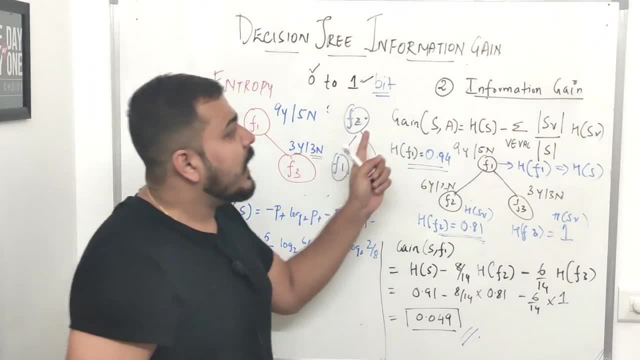 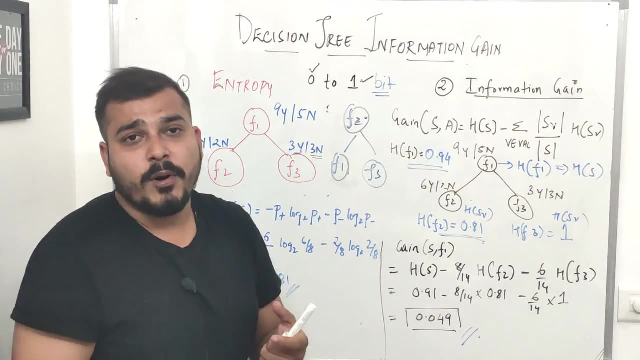 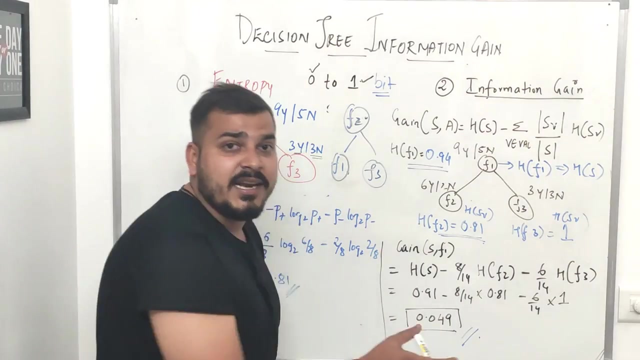 very, very important that you understand the entropic concept and you understand the information gain concept. now, guys, this particular formula you need to remember sometimes it is pretty much important. i know decision tree algorithm will do it automatically, which, whichever split it is doing, it will try to calculate the information gain considering the entropy in mind. 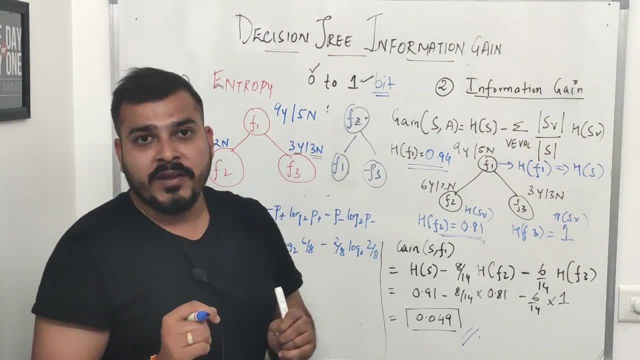 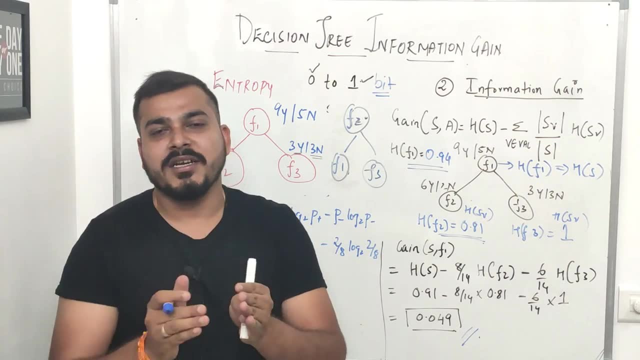 but here we need to understand how these specific things work, and this is how it actually works. many of you had this particular question, krish, why you're not uploading information gain. i'm extremely sorry. did you try and crush? i was not able to do it, but now you will be able to understand. 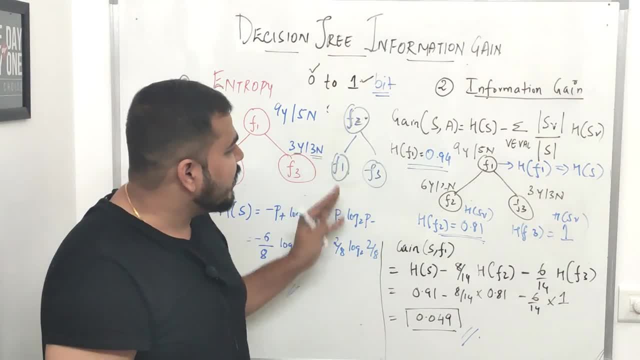 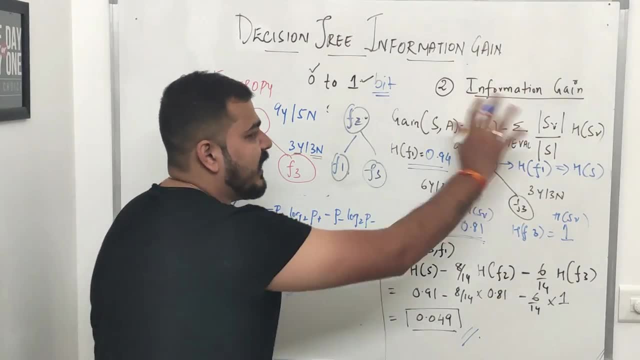 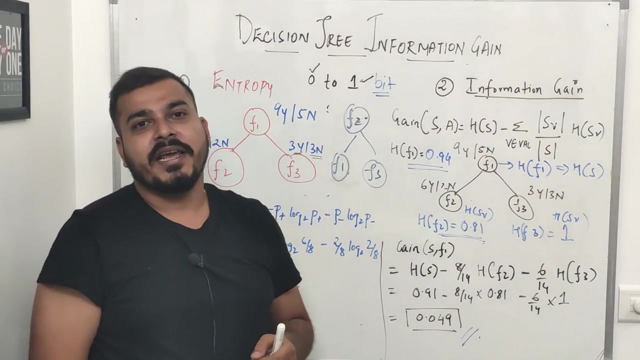 it okay. so finally, you can understand that whichever decision- and this can be any number of this uh splits that we can have, the total information gain will be computed. whichever split, whichever different, different types of splits are there which are having the highest information gain, that kind of structure of that decision tree will be taken up and that is how the training actually.